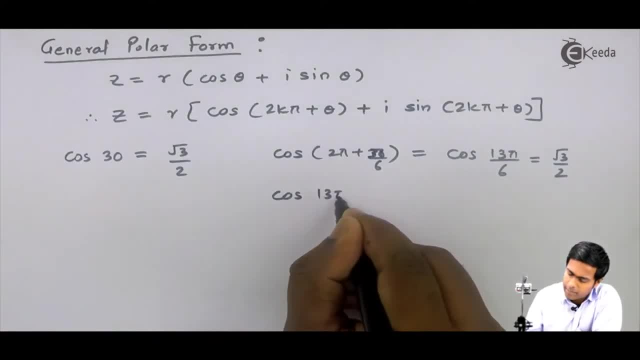 then let's try to find it manually. So let's try to find out the value of cos of 13 pi by 6.. So let's try. cos of 13 pi by 6 is equivalent to cos of pi plus, or I can say 2 pi plus pi by 6.. 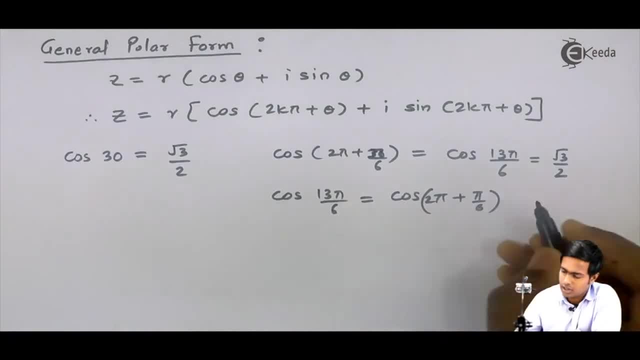 Now, cos of 2 pi plus theta is cos theta, So I will get cos of pi by 6, and cos of pi by 6 is root 3 by 2.. Similarly, if I will add 4 pi in this 30 degree, then I will get cos of pi by 6.. 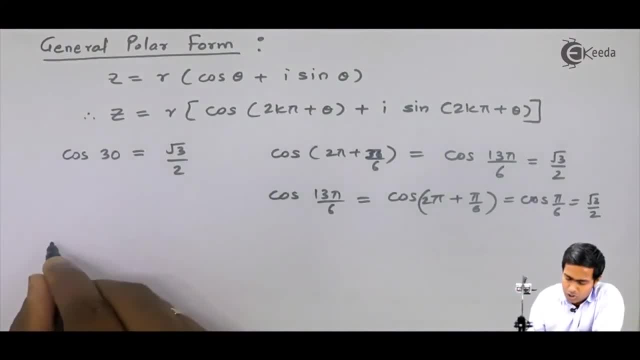 In this 30 degree, that is pi by 6, let's see what happens. So cos of 4 pi plus 30, that is pi by 6, will give me again cos of pi by 6, because cos of 4 pi plus theta is cos of theta. 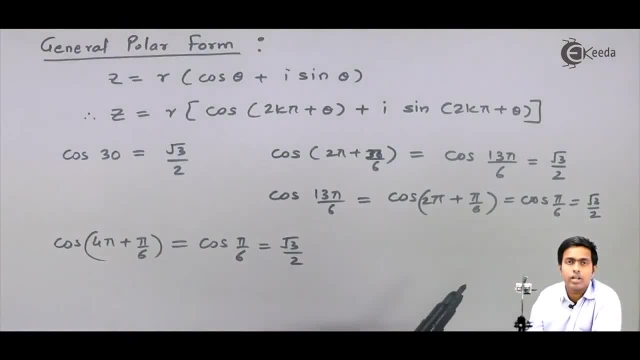 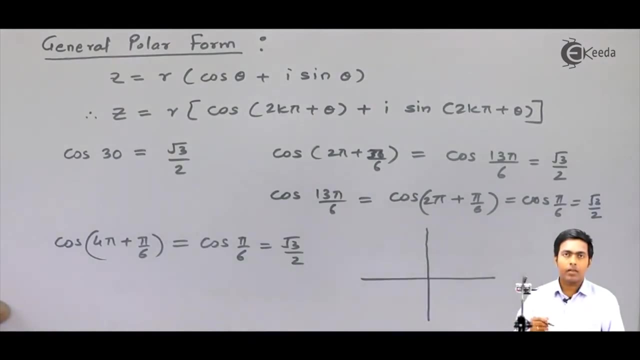 and it will again give me root 3 by 2.. So here you can observe that after every 2 pi angle we reach at the same point. We can also understand this concept from the diagram. Let's consider this. Let's say the angle is 30 degree. It means the point can be at. 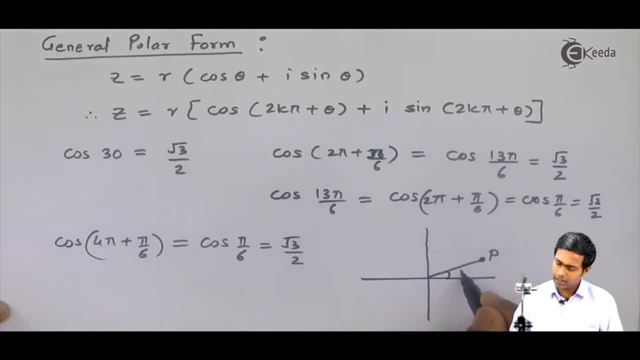 this place. So this is angle 30. So when I am adding 2 pi in it, 2 pi is nothing but 360 degree. So after moving 360 degree I am again reaching at the same point When I add 4 pi, 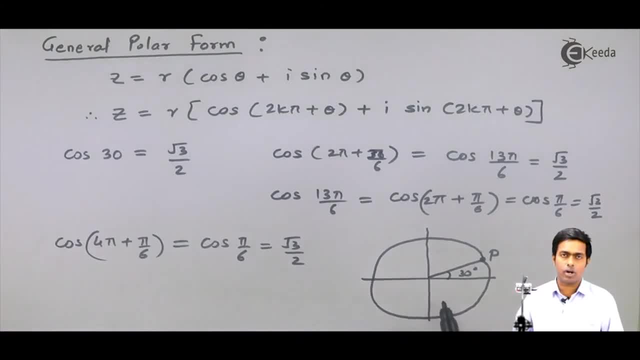 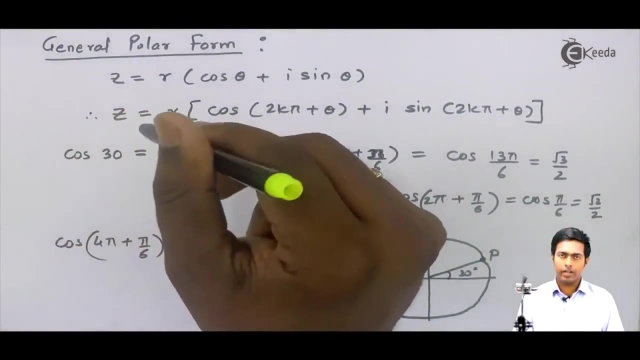 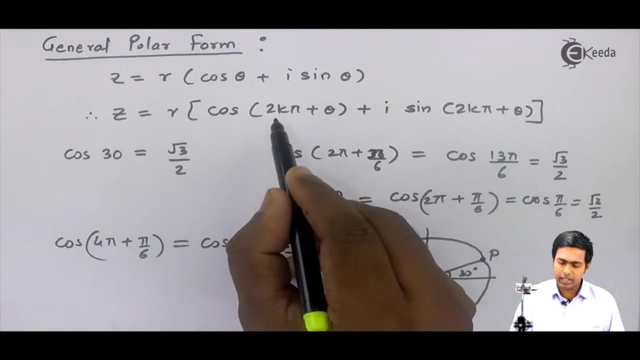 I again move 360 degree more, or I will say I move 720 degree. So after moving 720 degree I again reach at the same point. So every time we get the same answer. So general polar form: we generally find out by adding multiple of 2 pi in the amplitude. So hence I have represented. 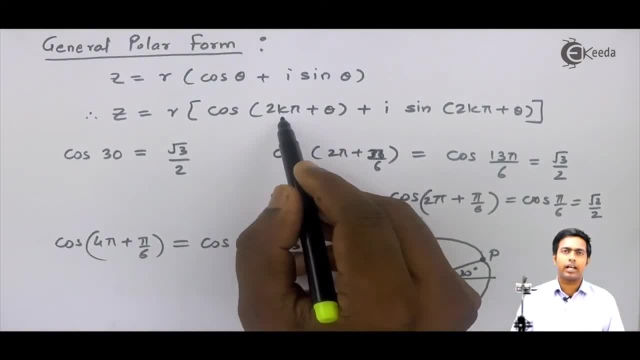 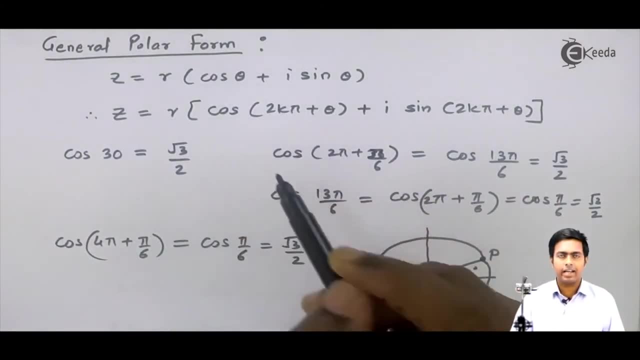 as 2 k pi, where k is integer, So it can take values as 1,, 2,, 3,, 4,, 5, 6 and so on. So by adding 2 k pi in amplitude we can get general polar form. So